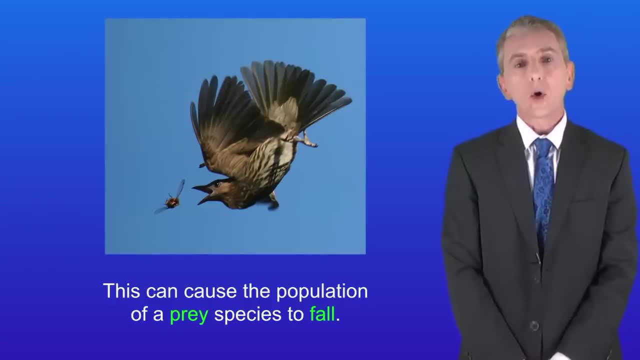 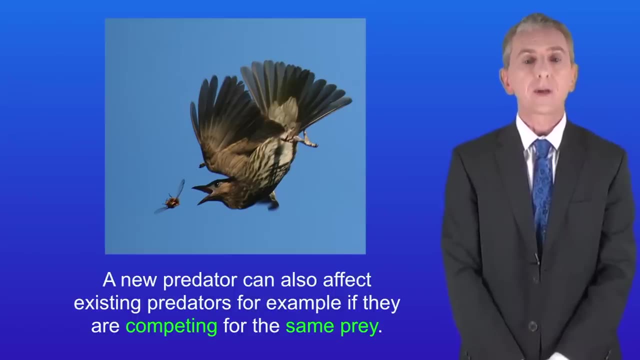 biotic factor is the availability of food. The number of organisms in that community is the arrival of a new predator. This can cause the population of a prey species to fall. A new predator can also affect existing predators, for example if they're competing. 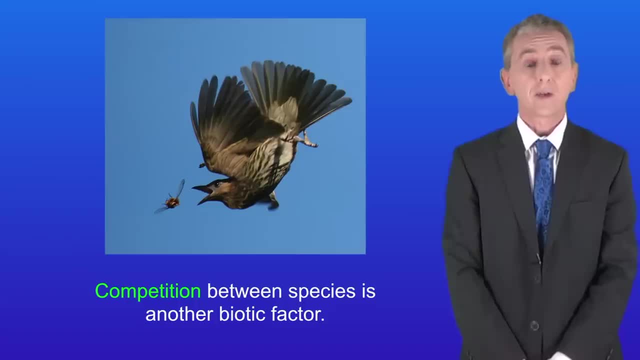 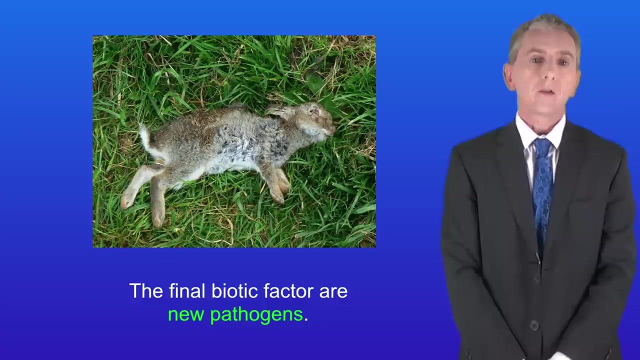 for the same prey. Competition between species is another biotic factor. If a species is out-competed, then its population can fall so much that numbers are no longer sufficient to breed and the species may become extinct. The final biotic factor are new pathogens. 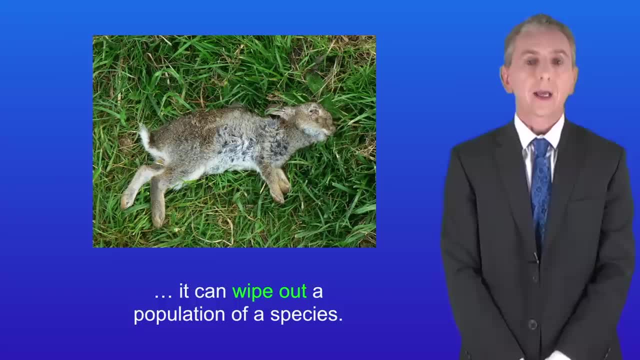 If an infectious disease emerges and then spreads, it can wipe out a population of a species. Okay, we're going to take a look now at abiotic factors, and remember that abiotic means not living. There are seven different abiotic factors and in the exam you could 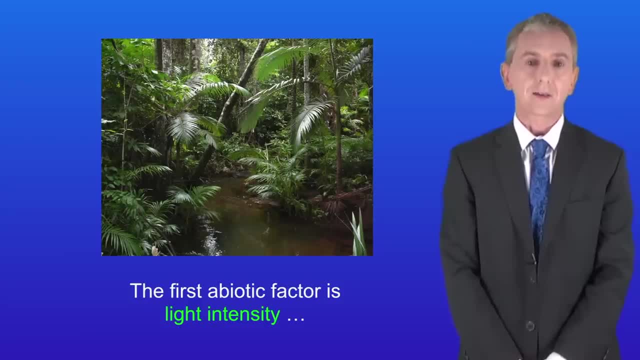 be asked about any of them. The first abiotic factor is light intensity, and this can have a major effect on plants. All plants need light to carry out photosynthesis. However, if the light intensity is too low, then the rate of photosynthesis falls and plants will grow. 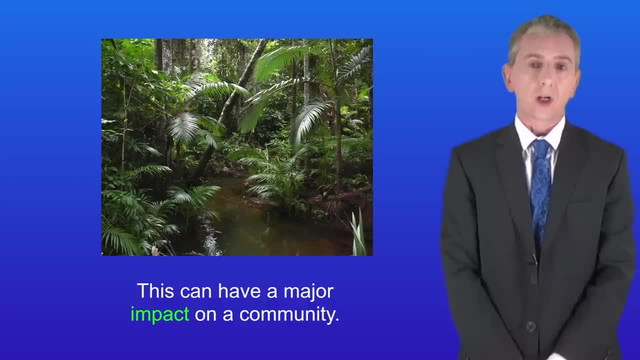 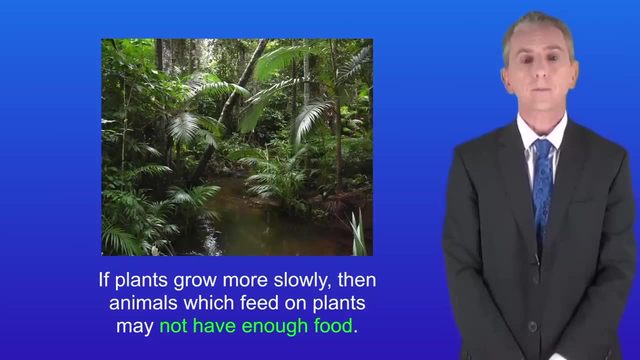 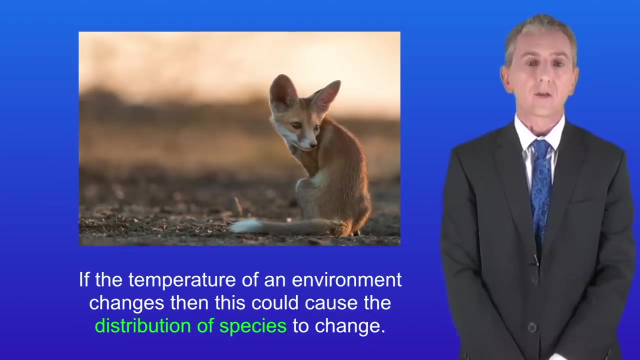 more slowly. Now this can have a major impact on a community. If plants grow more slowly, then animals which feed on plants may not have enough food. Temperature is also a really important abiotic factor. If the temperature of an environment changes, then this could. 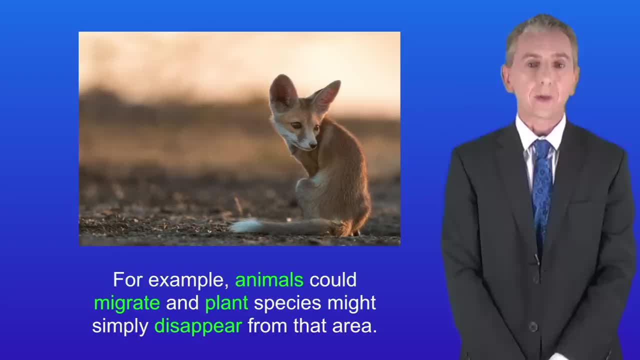 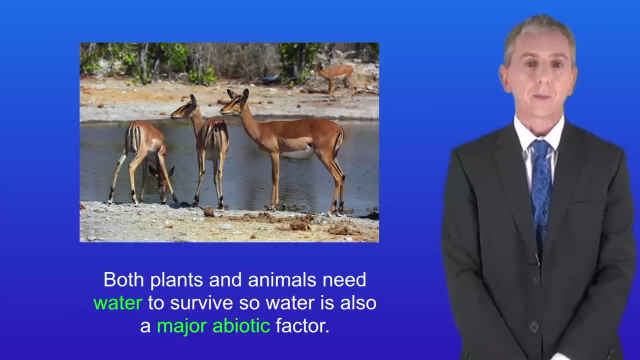 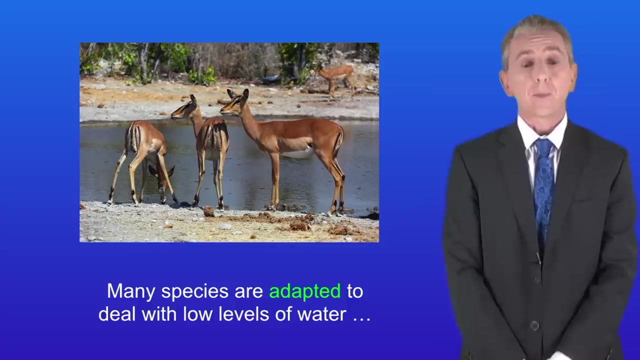 cause the distribution of species to change. For example, animals could migrate and plant species might simply disappear. Both plants and animals need water to survive, so water is also a major abiotic factor. Many species are adapted to deal with low levels of water, and we'll be looking at these adaptations. 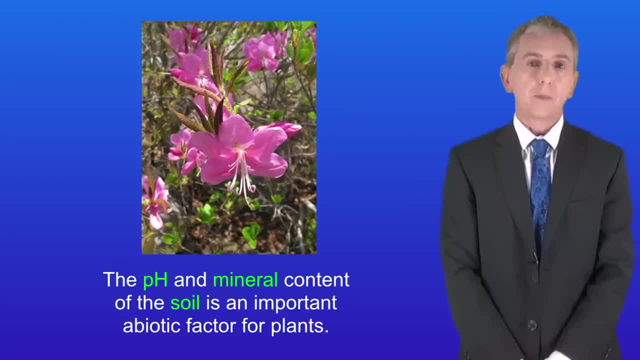 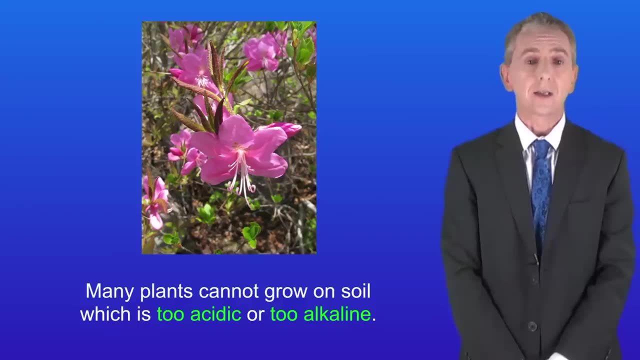 in the next video. The pH and mineral content of the soil is an important abiotic factor for plants. Many plants cannot grow on soil which is too acidic or too alkaline. Plants also need certain minerals in the soil, For example nitrate, which is used to make amino acids for proteins.